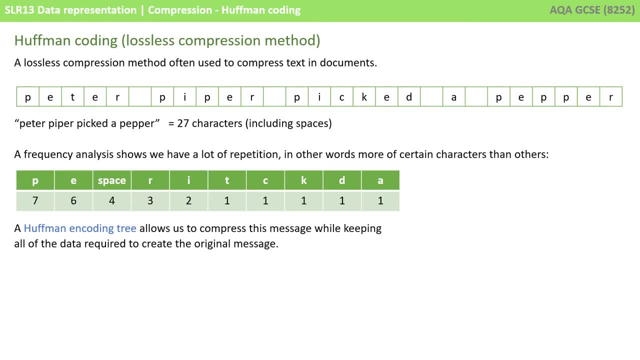 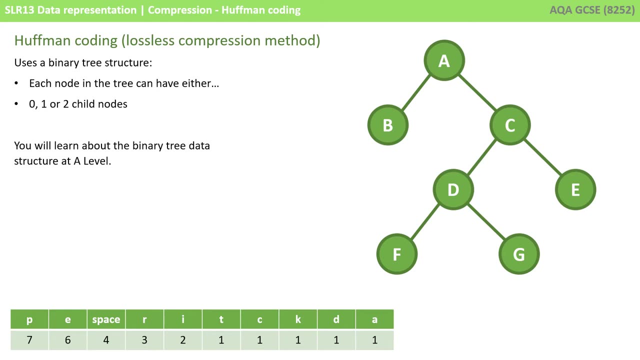 encoding tree allows us to compress this message while keeping all of the data required to recreate the original message. So Huffman coding makes use of what are known as binary trees. Now, this is a data structure that you'll learn about at A level. All you need to know is that, with 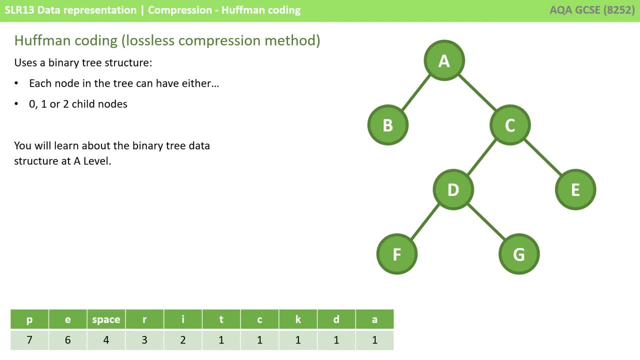 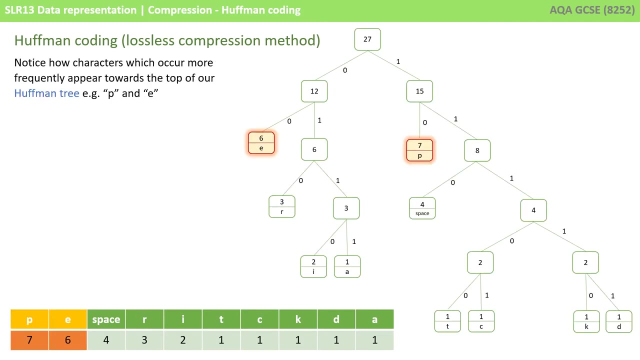 binary trees. we have nodes, and each of those nodes can have not one or two child nodes, but no more than two, Hence the term binary tree. So here is the Huffman coding tree for the phrase we looked at earlier. Now you don't need to create these in the exam, but notice how. 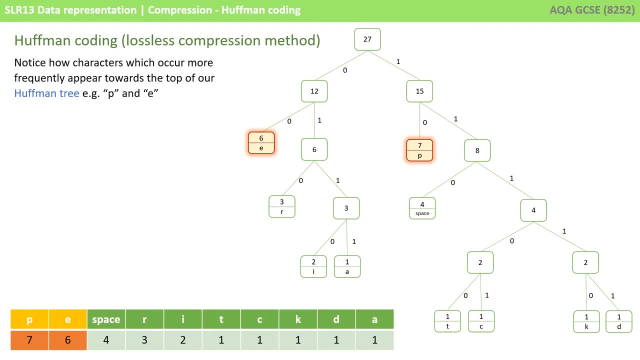 characters which occur more frequently are appearing towards the top of a Huffman tree. So P and E, which had seven and six occurrences each, are quite close to the top of a Huffman tree, Whereas characters which occur less frequently, by the letter T and C, which appear only once, appear towards the bottom of our Huffman tree. 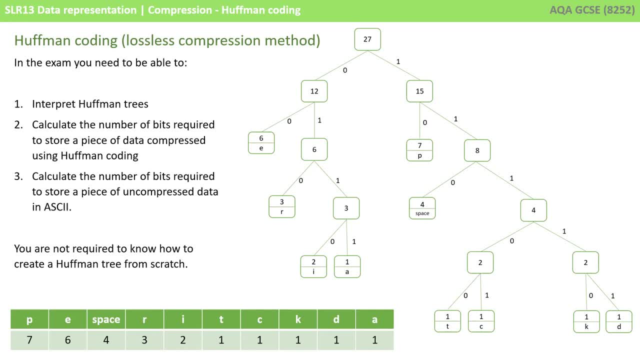 So, as just mentioned, you're not going to be required to know how to create a Huffman tree from scratch in the exams, but what you will need to be able to do is to be able to interpret a Huffman tree, calculate the number of bits required to. 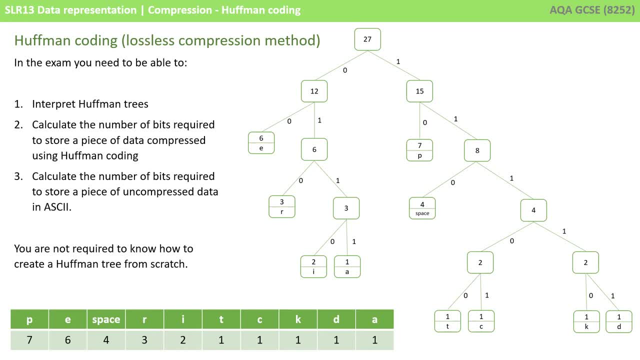 store a piece of data compressed using Huffman coding and calculate the number of bits required to store a piece of uncompressed data in ASCII and compare the two. So let's take a look at that now. So, given the Huffman tree shown here, how could the character P be encoded? Well, 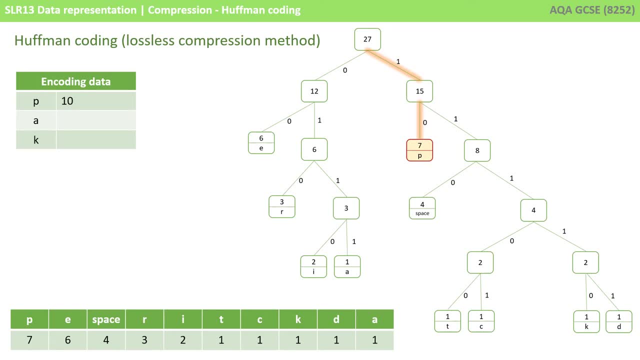 you can see that every branch in our binary tree is given a 0 or 1, depending whether we're branching left or we're branching right, So we can provide the path taken to reach the letter P. It's 1 followed by 0,, so branching right and then left, So 1, 0 can be encoded to represent the letter P. 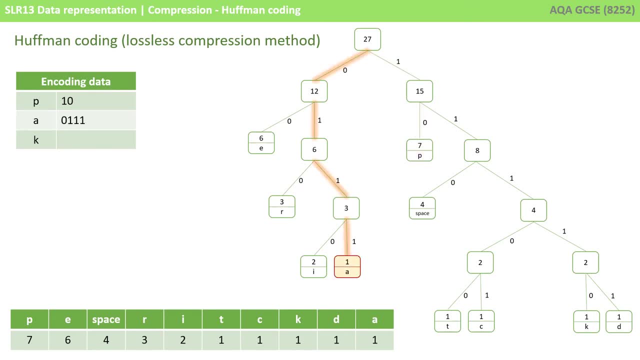 Now the letter A has a much longer encoding path. it's twice the size, it's 4 bits. To get to the letter A we have to follow the path 0, 1, 1.. In a similar fashion, the encoding path for the letter K is 1, 1, 1, 1, 0.. We're branching right. 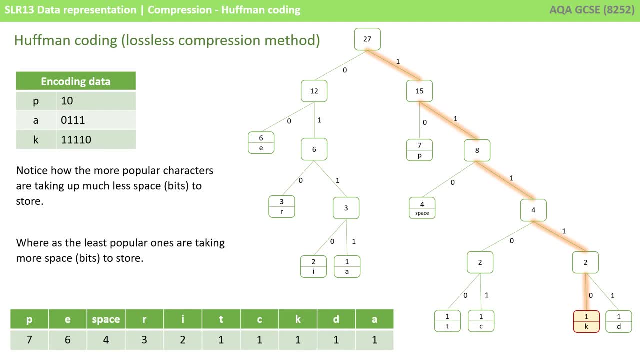 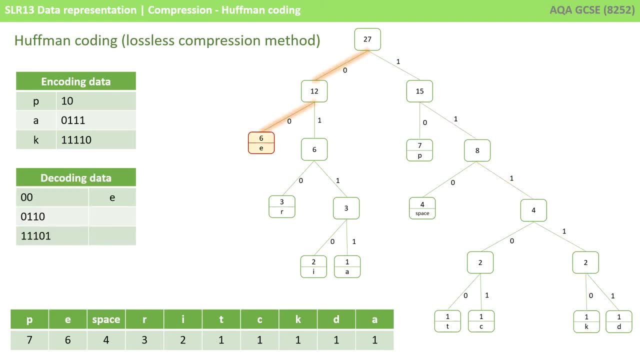 are taking up more bits, but that's okay, as we're using them less. are taking up more bits, but that's okay, as we're using them less frequently, as we're using them less frequently. as we're using them less frequently, You also need to be able to decode. 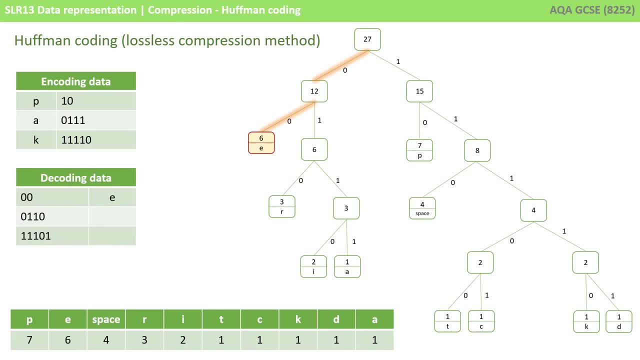 frequently. You also need to be able to decode frequently. You also need to be able to decode Huffman bit patterns from a Huffman. You also need to be able to decode Huffman bit patterns from a Huffman. You also need to be able to decode Huffman bit patterns from a Huffman tree you've been given. 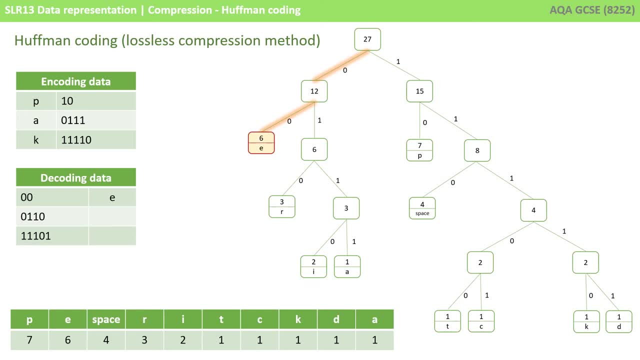 Huffman bit patterns from a Huffman tree. you've been given. Huffman bit patterns from a Huffman tree: you've been given. So if you were given the bit pattern tree, you've been given. So if you were given the bit pattern tree, you've been given. So if you were given the bit pattern, you start at the top, you follow. So if you were given the bit pattern, you start at the top, you follow. So if you were given the bit pattern, you start at the top, you follow the left branch zero and the left. you start at the top, you follow the left branch zero and the left. 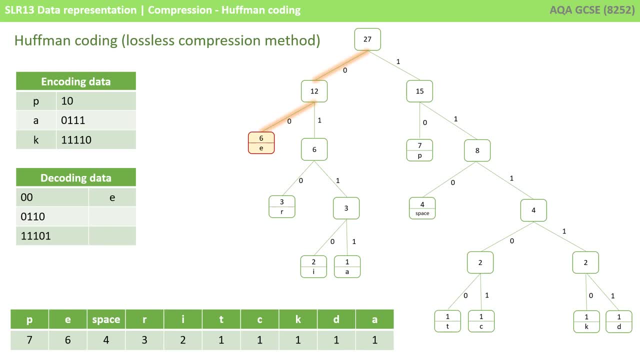 you start at the top, you follow the left branch zero and the left branch again zero, So that decodes the left branch zero and the left branch again zero. So that decodes the left branch zero and the left branch again zero. So that decodes into the letter E. 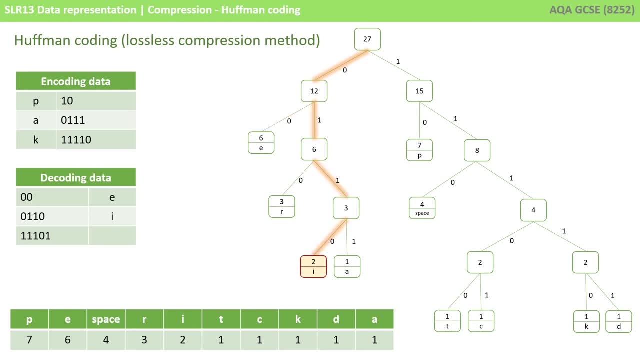 branch, again zero, So that decodes into the letter E branch, again zero, So that decodes into the letter E In a similar way: zero, one, one, zero. into the letter E In a similar way: zero, one, one, zero. 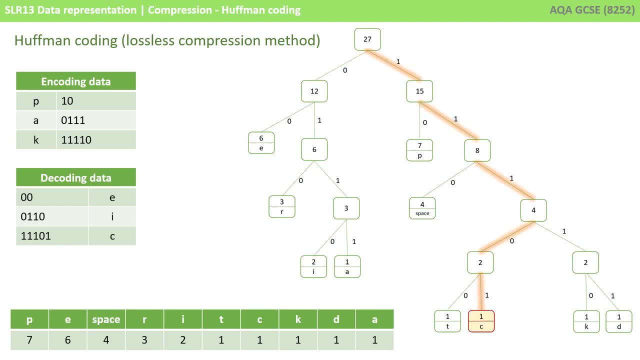 into the letter E. In a similar way, zero, one, one, zero one decodes into the letter I. In a similar way, zero, one, one, zero one decodes into the letter I. In a similar way, zero, one, one, zero one decodes into the letter I And one, one, one, zero one. 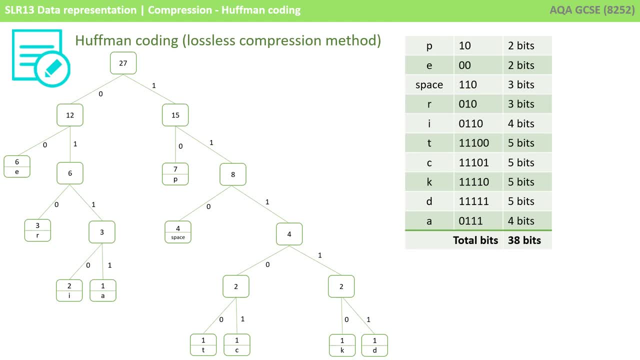 one, one, one, zero one decodes into the letter C. one, one, one, zero one decodes into the letter C. one, one, zero one decodes into the letter C. Now we've encoded each of our characters. into the letter C. Now we've encoded each of our characters into the letter C. Now we've encoded each of our characters using the Huffman tree, and we've worked. Now we've encoded each of our characters using the Huffman tree, and we've worked. 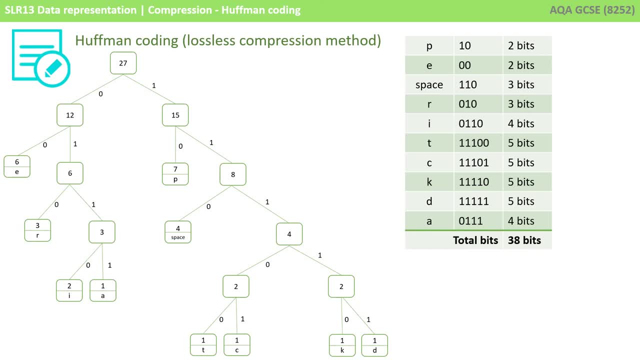 Now we've encoded each of our characters using the Huffman tree and we've worked out how many bits it's going to using the Huffman tree, and we've worked out how many bits it's going to using the Huffman tree and we've worked out how many bits it's going to take to store each character. 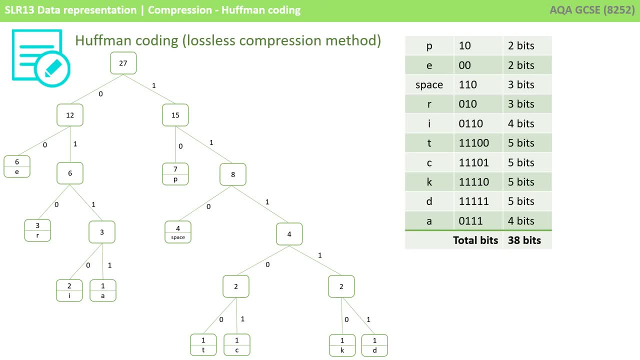 out how many bits it's going to take to store each character. out how many bits it's going to take to store each character. We almost have all the information take to store each character. We almost have all the information take to store each character. We almost have all the information we need to work out how much space. 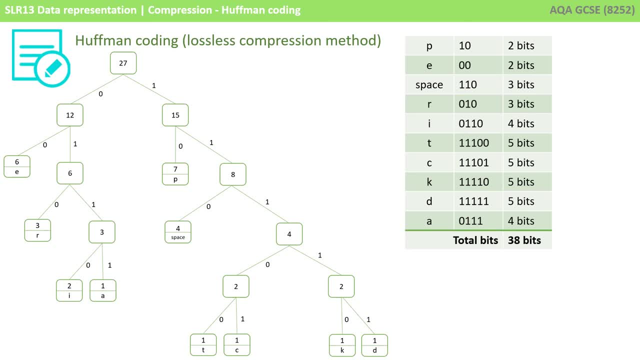 We almost have all the information we need to work out how much space. We almost have all the information we need to work out how much space we have saved using this method. we need to work out how much space we have saved using this method. we need to work out how much space we have saved using this method of compression So we can see that. we have saved using this method of compression. So we can see that we have saved using this method of compression. So we can see that p takes two bits to encode a one of compression. So we can see that p takes two bits to encode a one. 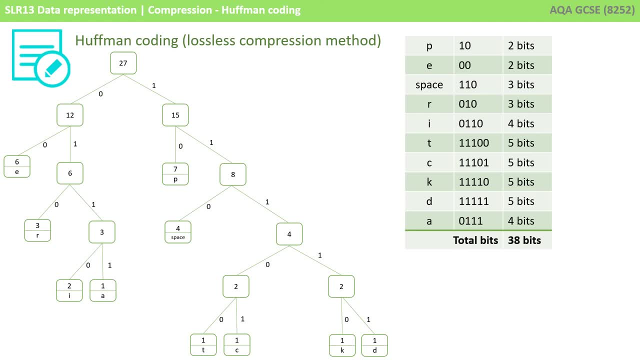 of compression. So we can see that p takes two bits to encode a one and a zero, whereas an i takes. p takes two bits to encode a one and a zero, whereas an i takes. p takes two bits to encode a one and a zero, whereas an. i takes four bits to encode zero, one, one, zero. 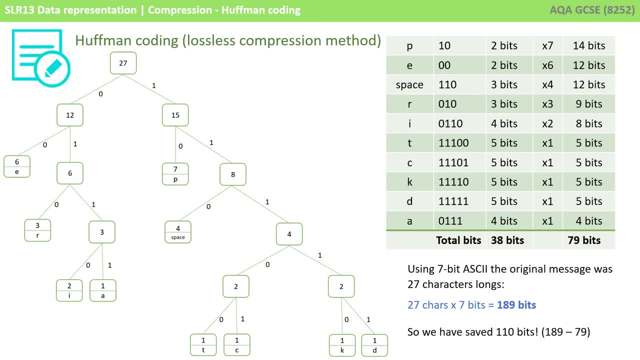 Of course we also need to take into, Of course we also need to take into, Of course we also need to take into account the frequency with which each account, the frequency with which each account, the frequency with which each character appears, So, although the character appears, So although the 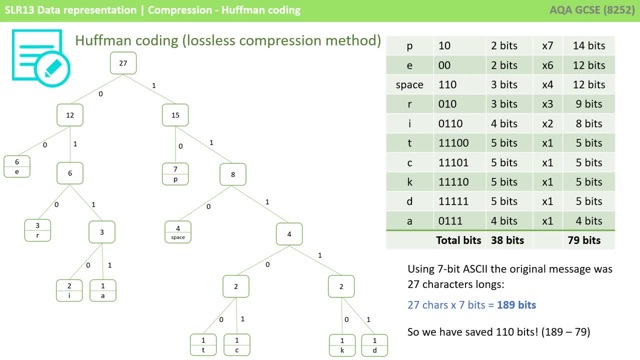 character appears. So, although the character p, character p, character p takes two bits to encode a one and a zero, takes two bits to encode a one and a zero, takes two bits to encode a one and a zero. there are seven occurrences of the. there are seven occurrences of the. 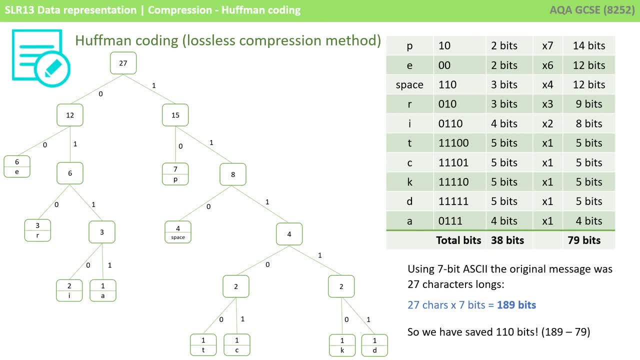 there are seven occurrences of the character p, character p, character p. therefore, this is 2 times 7 or 14 bits. therefore, this is 2 times 7 or 14 bits. therefore, this is 2 times 7 or 14 bits. this gives us a total of 79 bits to. 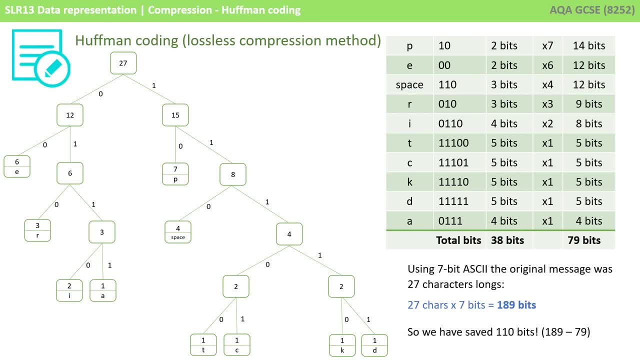 this gives us a total of 79 bits to. this gives us a total of 79 bits. to encode this message using Huffman. encode this message using Huffman. encode this message using Huffman encoding encoding: encoding: Now using normal 7-bit ASCII: the: Now using normal 7-bit ASCII: the. 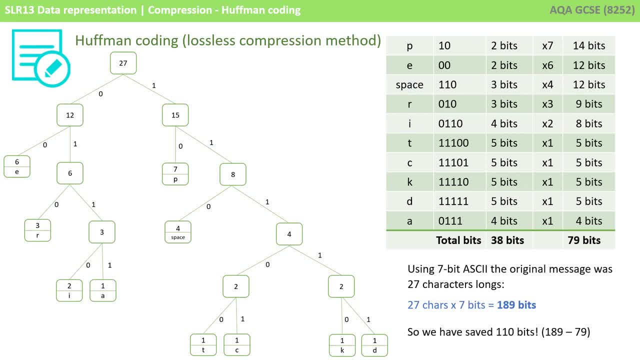 Now using normal 7-bit ASCII. the original message was 27 characters long. original message was 27 characters long. original message was 27 characters long. so that would have been 27 characters. so that would have been 27 characters. so that would have been 27 characters times 7 bits for characters and 189. 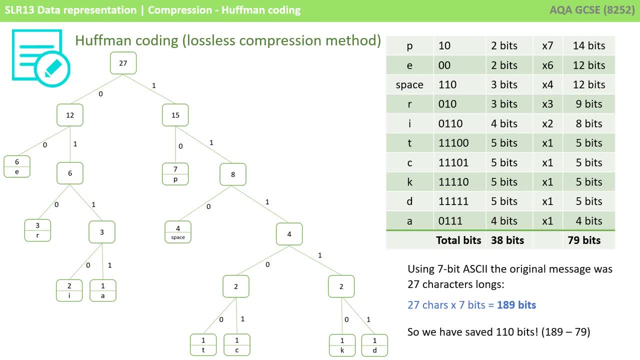 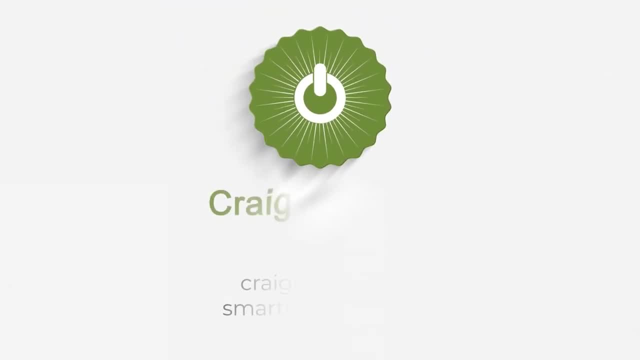 times 7 bits for characters and 189 times 7 bits for characters and 189 bits, bits, bits. So we've saved 110 bits. So we've saved 110 bits. So we've saved 110 bits by using Huffman coding. So we've saved 110 bits by using Huffman coding. 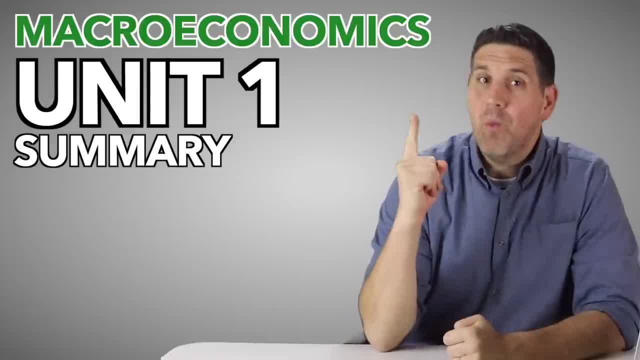 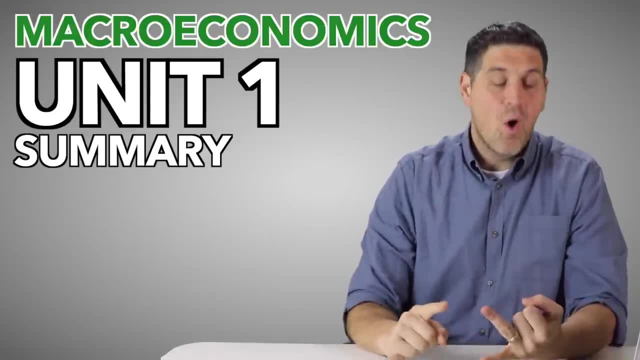 Hey econ students, this is Jacob Clifford. Welcome to the macroeconomics unit. one summary video. Now, in the summary videos I explain all the concepts over again to get them back in your brain, to get you ready for your exam or the final exam, or your midterm or the AP test. I'm going to get you. 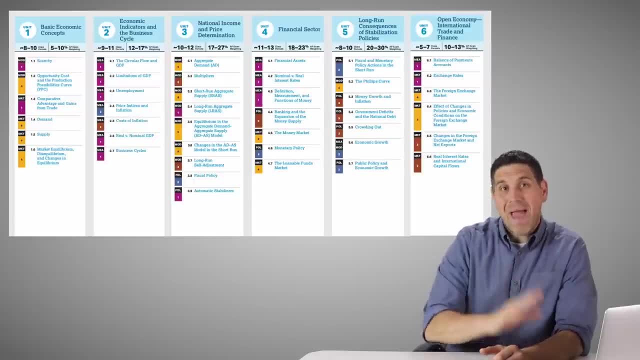 everything you need really quick. I've organized this course based on the AP macroeconomics curriculum, but keep in mind, if you're in college or even a master's program, if you're learning macroeconomics. all the key concepts are in here, And be sure to check out my ultimate review packet. 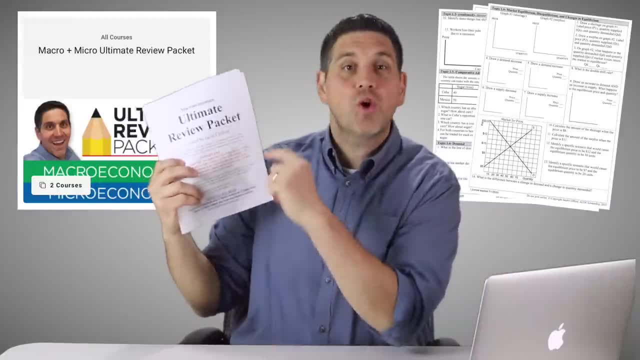 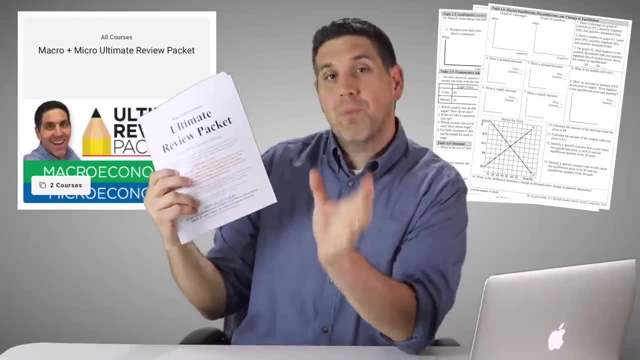 It goes along with these videos and includes tons of practice. So, as you're watching this video, fill out the blank unit study guide, then check your answers to verify. you can do the calculations and draw different graphs. and make sure to do the practice tests and watch the exclusive videos. 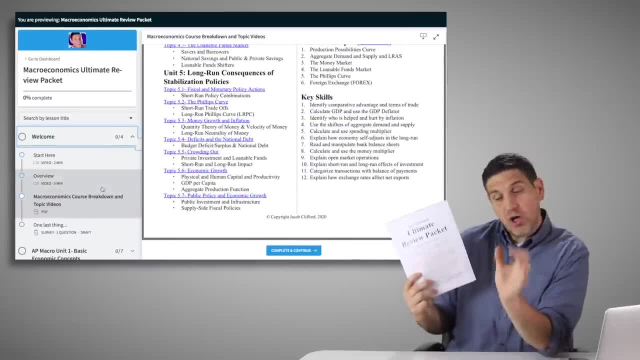 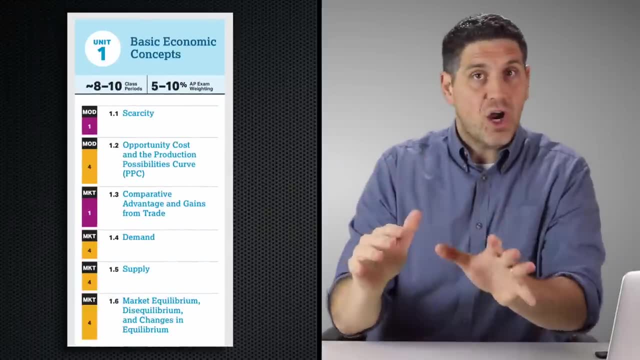 that are all part of the pack, And the first unit is free, So make sure to go download the unit one study guide and fill it out as you're watching the rest of this video. Okay, here we go. Macroeconomics unit one. It all starts with the basic economic concepts, So we're starting off with scarcity. 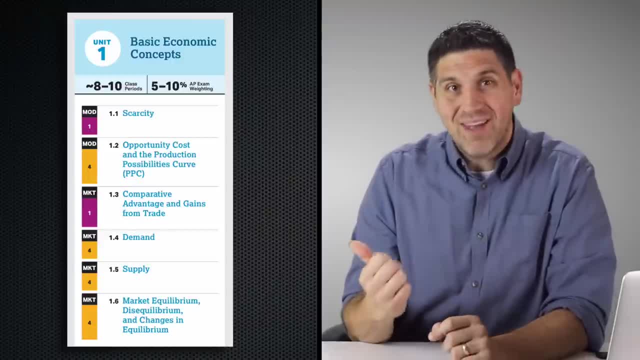 opportunity, costs and the production possibly is curve. Then we'll talk about comparison and cost, And then we'll talk about the cost of production, And then we'll talk about advantage and trade, then demand, supply and putting supply and demand together and finding.